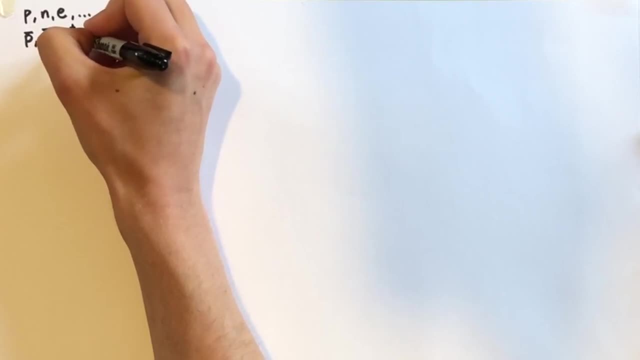 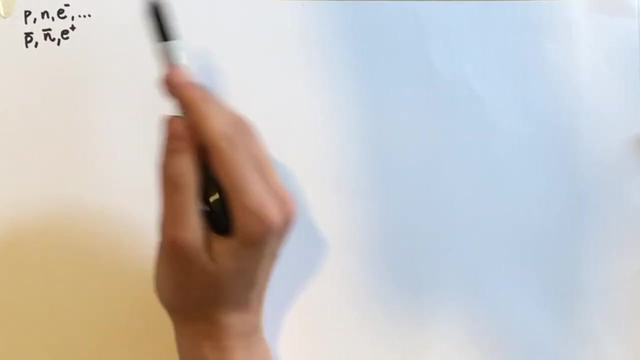 actually known as the positron, which we write with a little e plus right here. It should be a little minus there to show that the electron is negatively charged and the positron is positively charged. So the only difference between particles and antiparticles is that they have opposite. 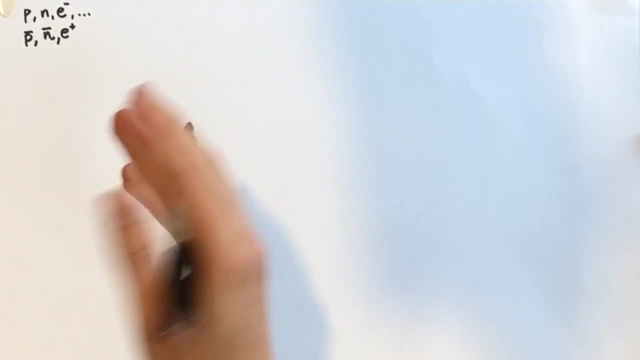 charge to that of their corresponding particle. Everything else about them is the same. they have the same mass and they have the same other particle properties, which we'll have a look at more in future videos. Now, when particles and antiparticles collide, they will annihilate and emit radiation. So say we. 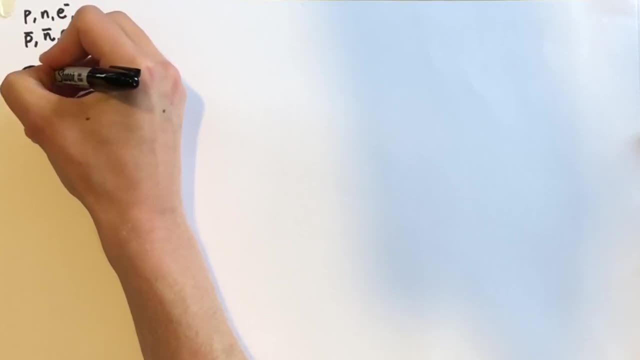 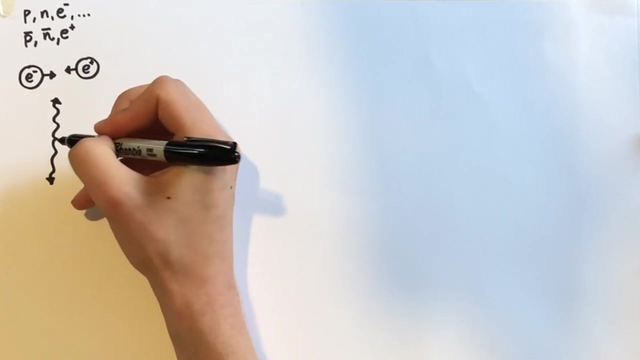 have an electron and a positron and say they're heading towards each other, and when they hit each other and collide, they will annihilate and produce, release energy. that's in the form of electromagnetic radiation, and this electromagnetic radiation is normally in the gamma range, part of the 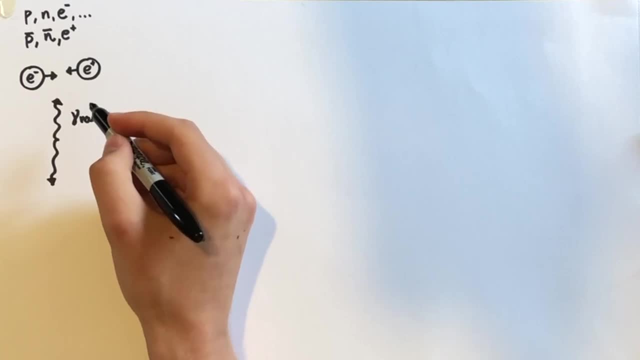 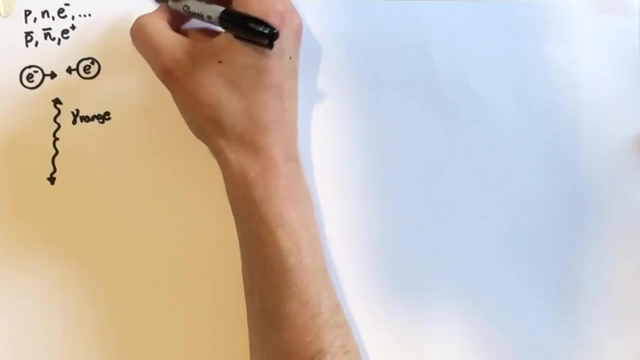 spectrum. You can actually produce these positrons by what's known as beta plus decay. In the last video I mentioned beta minus decay, in which you have a neutron, a proton, a neutron and a neutron, So you have a neutron that turns into a proton. 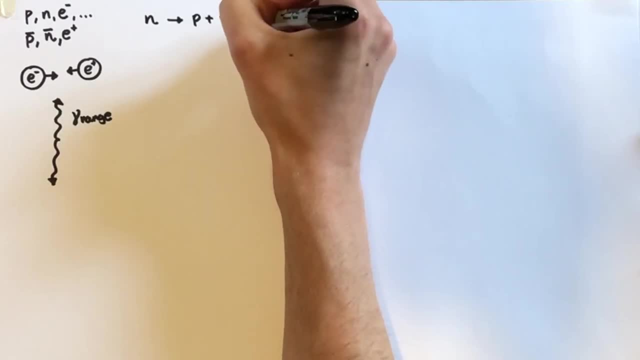 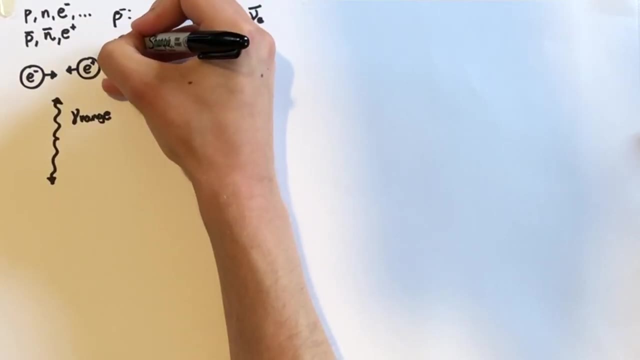 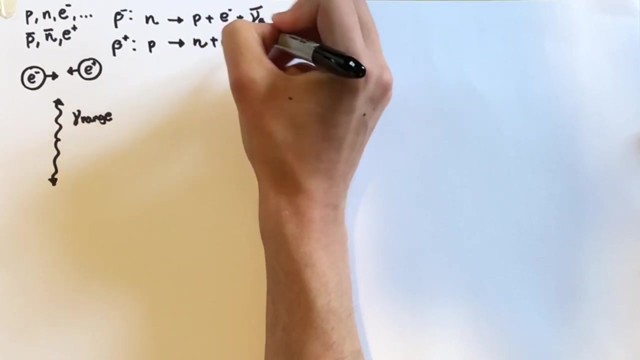 plus an electron, plus an electron anti neutrino. So that's basically the standard equation for beta minus decay. Now, beta plus decay, actually almost the opposite happens. You have a proton changing into a neutron, but instead of releasing the electron, you actually get a positron. and instead of an anti-electron neutrino, you actually 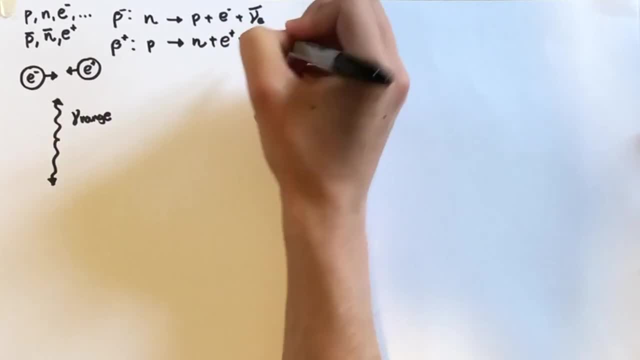 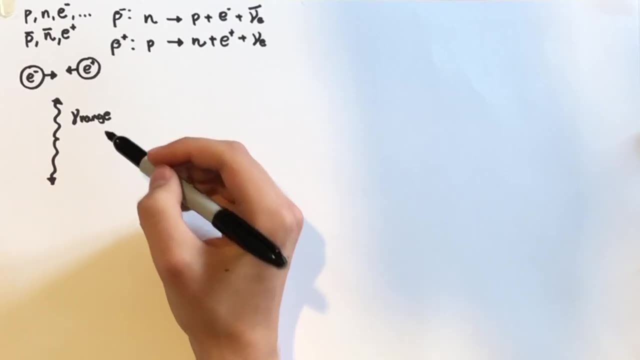 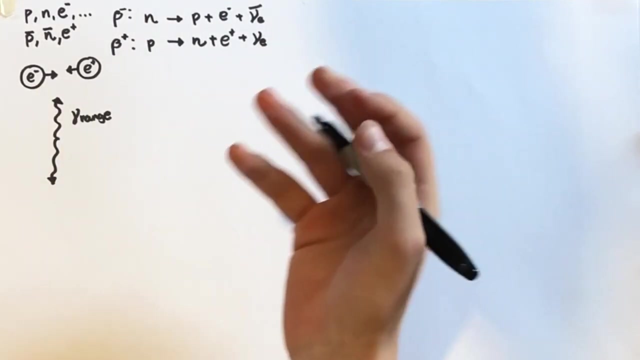 get just a normal electron neutrino Now. antimatter was first predicted in 1928 by the English physicist Paul Dirac in his famous equation known as the Dirac equation. Now Dirac equation is quite a long and complicated equation, so thankfully you don't need to know it for A. 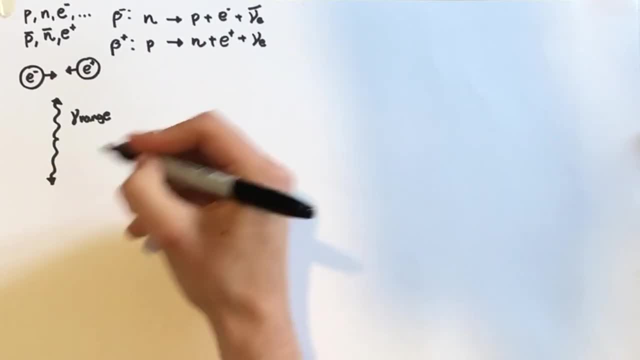 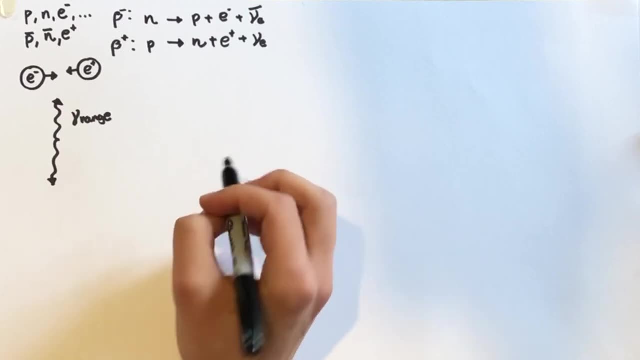 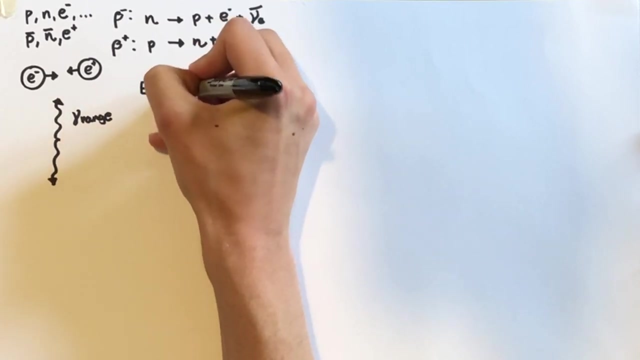 level, But antimatter then went on to be discovered a little while afterwards, after it had been predicted. However, before then, it was Einstein that showed that energy and mass were linked by his famous equation E equals MC squared, which said that there was a large amount of energy locked away in a small mass. 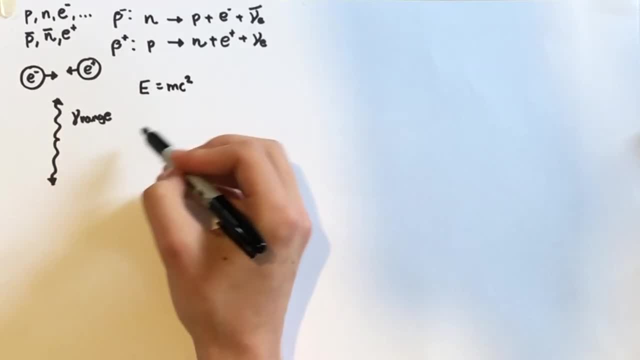 and it's that energy that gets released in the form of a gamma-ray photon when a particle and an anti-particle collide. So let's draw a diagram of this. So you have an electron and a positron that are colliding, so they're moving towards each other, and when 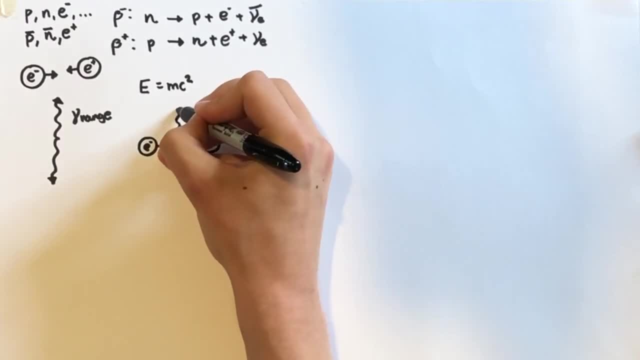 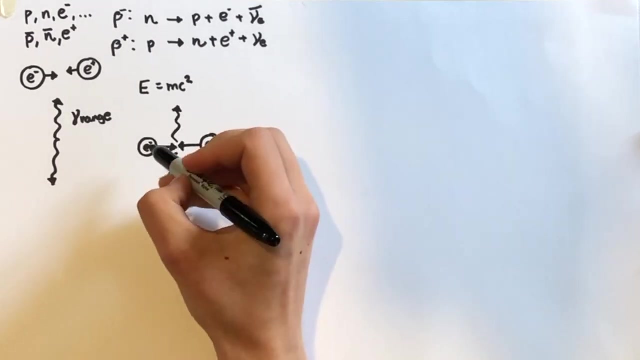 they move towards each other. they actually produce two gamma-ray photons, от и, And the energy of these two gamma-ray photons combined is equal to the energy that corresponds to these two electrons, which is locked up in the form of their mass. So electrons, of course, are really really light particles. 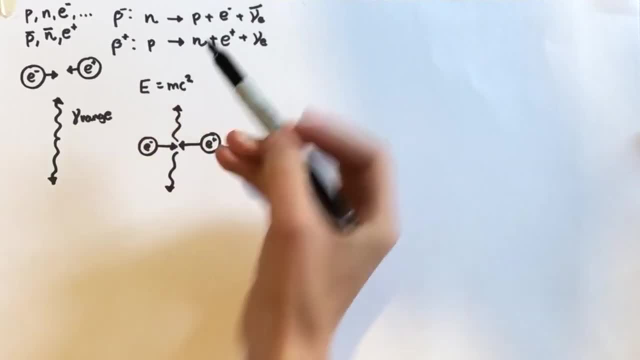 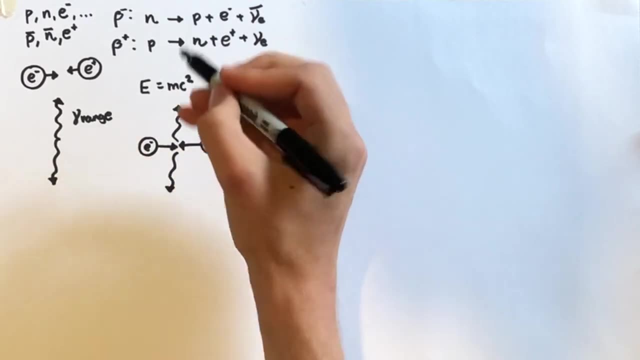 But because there's so much energy per unit mass, because of course they're linked by this constant here, which is the speed of light squared. The speed of light was a massive number, of course, but the speed of light squared is going to be what? 9 times 10 to the 16,. 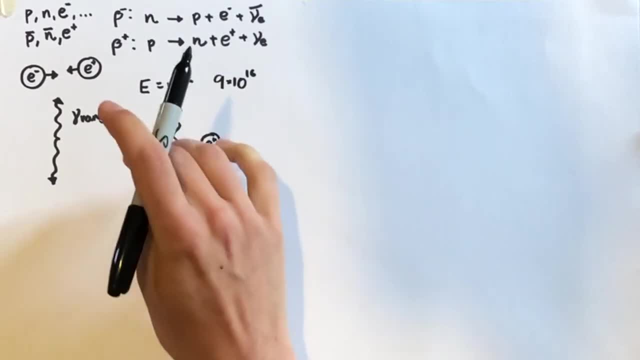 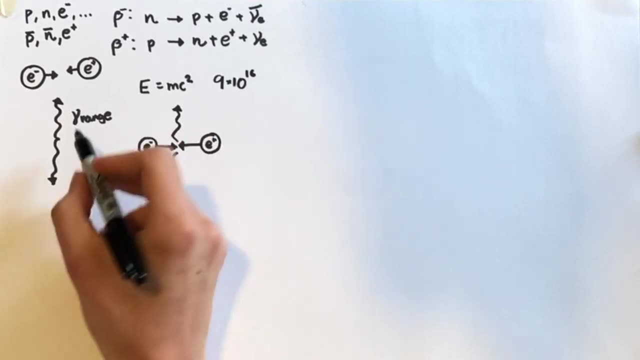 just 3 times 10 to the a squared, You're going to get a humongous amount of energy being released from these two particles, And so that's why it's in the gamma range of the spectrum. But we can also consider this the other way around, in which, rather than mass gets converted into energy. 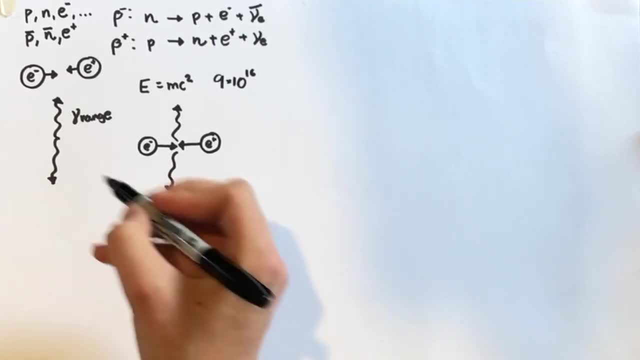 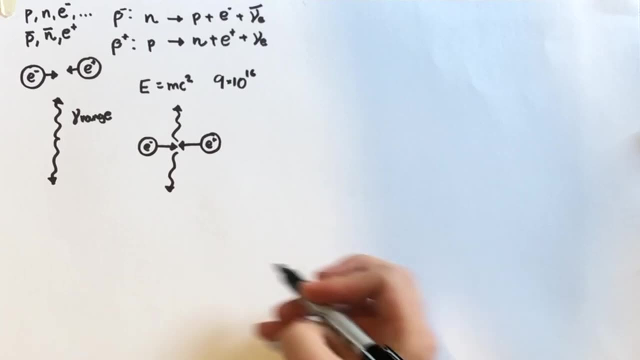 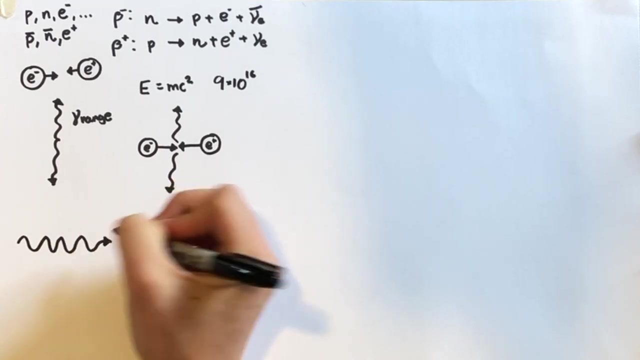 we can have energy, Energy in the form of electromagnetic radiation being converted into mass, And this we refer to as pair production, So say we have a high energy, high energy gamma ray. Now that will actually turn into two particles, one of which. 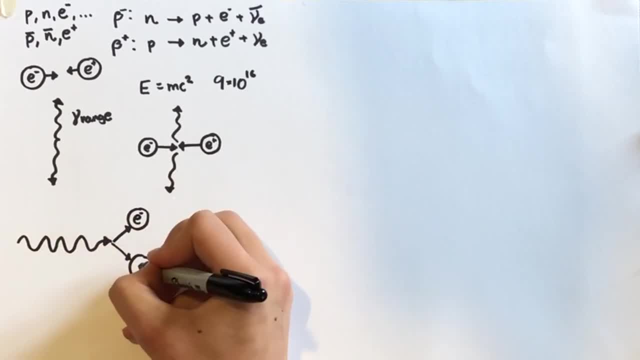 One of which is An electron and one of which is a positron, and you always get it like this: You could, you can't- create matter without antimatter. It always happens in pairs. Now, a lot of the time in physics, you may see that some of the energies that we're talking about here are not given in the standard SI unit of Joules. 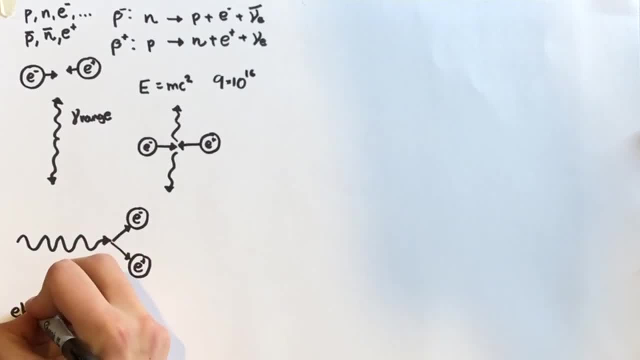 but rather in this funny unit called electron volts. So what's an electron volt? Well, an electron volt is It is defined. it is defined as the energy needed to an accelerate to accelerate an electron through a potential difference of one volt. 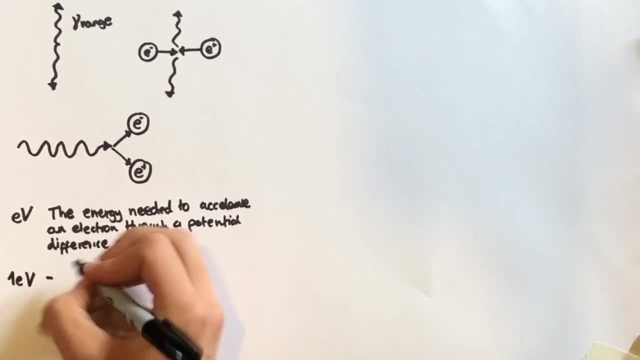 And one electron volt is exactly the same as saying 1.6 times 10 to the minus 19 Joules. Now you might recognise this number right here: 1.6 times 10 to the minus 19. And this is the charge on an electron. 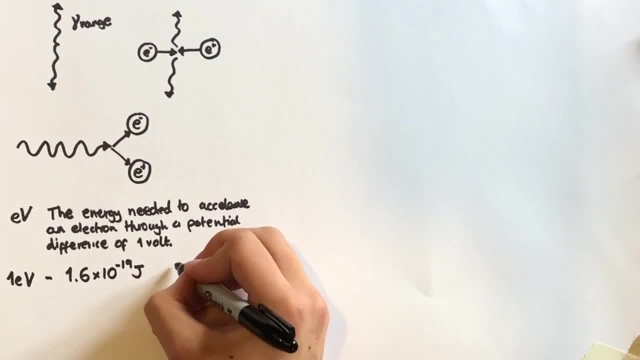 Now later on in the course, there is an equation Which states that energy equals charge times the voltage, And that's quite a big equation in A-level physics and that's basically saying that charge is the energy per unit volt. So if you have 1.6 times 10 to the minus 19 Coulombs multiplied by a potential difference of one volt, 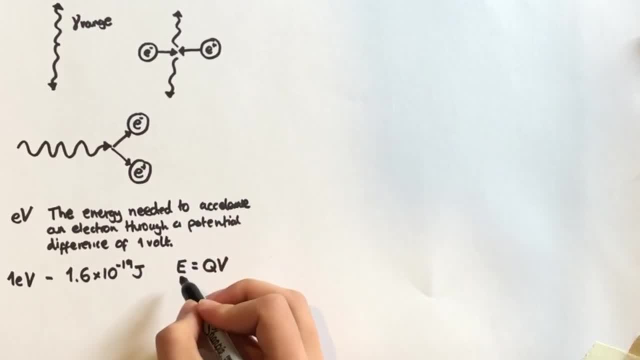 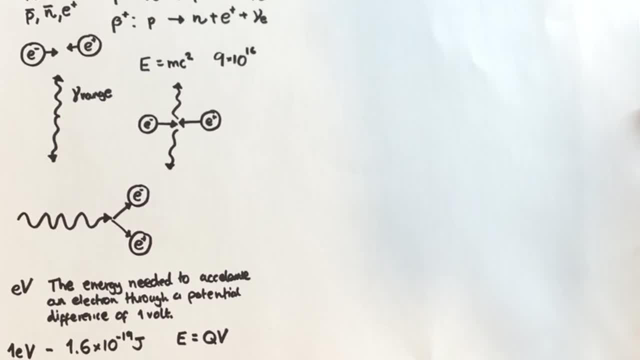 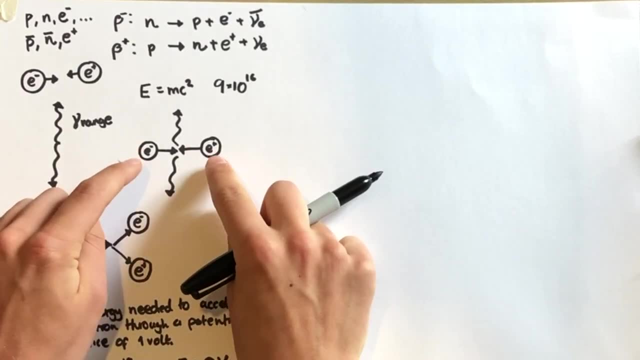 which is the same as an electron volt, which is the same as an electron volt, which is the same as an electron volt. So now let's consider the energies involved in annihilation and pair production. In annihilation, we've got the two particles which, from Einstein's equation, have what's known as rest energies. 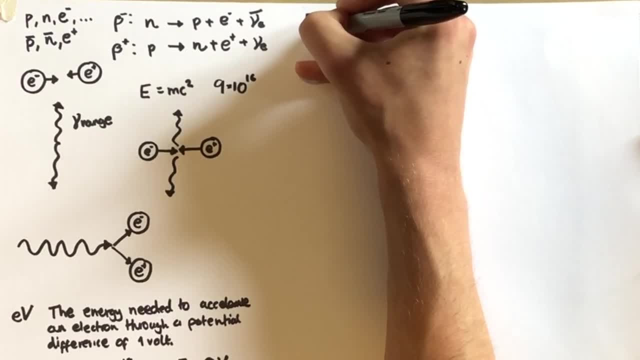 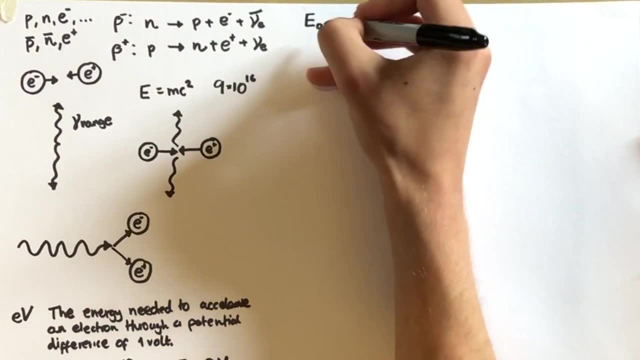 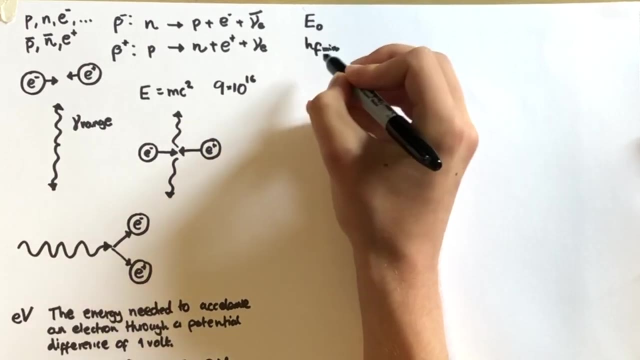 We normally denote rest energy by the little term E0.. Now these two particles will then annihilate and produce two photons which have energy Hf, which have energy Hf, And Fmin is the minimum frequency We can equate these two energies, saying that 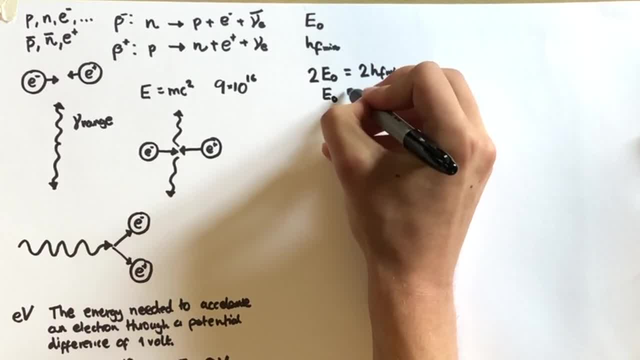 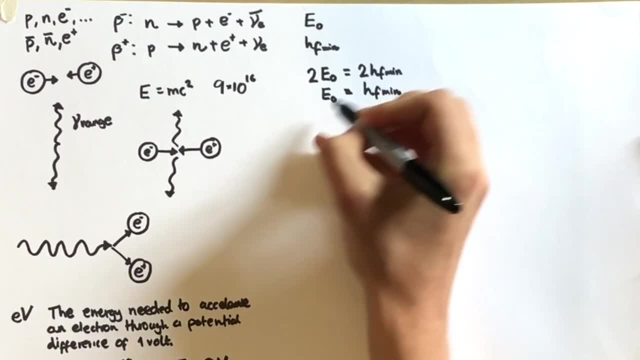 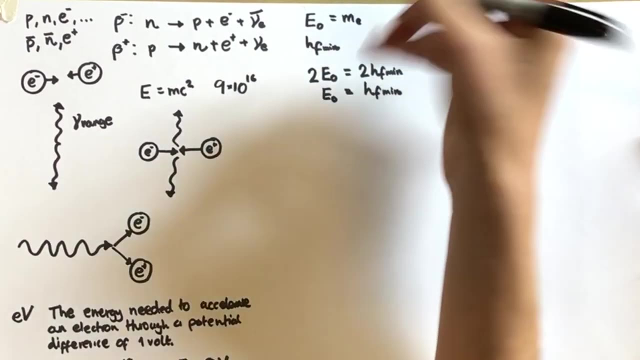 And if we divide both sides by two, we get that h f min, Whereas E naught is simply E naught equals m, mass of the particle. in this case we're dealing with an electron times the speed of light squared. That is the rest energy. 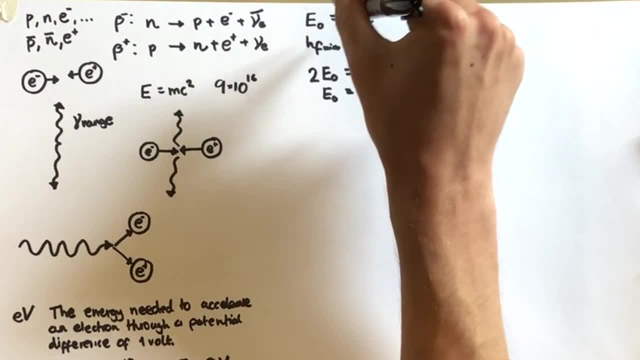 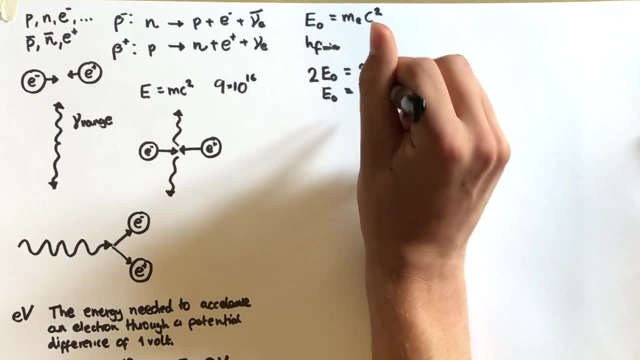 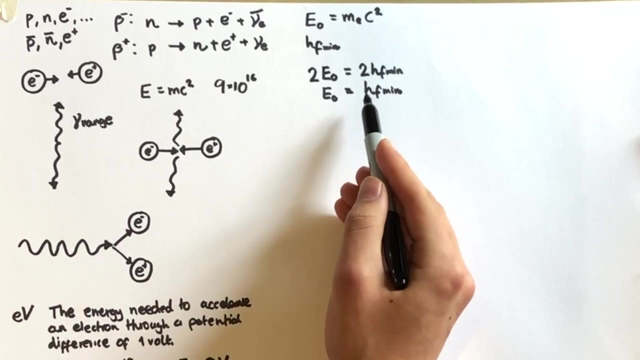 It's the energy that's locked up within an electron due to its mass And that corresponds to a frequency f min. And that minimum frequency is normally in the gamma ray part of the spectrum, which is why you need radiation with enough energy to get to this. rest energy here. 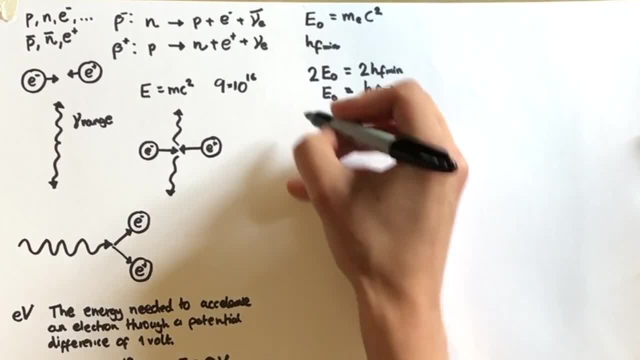 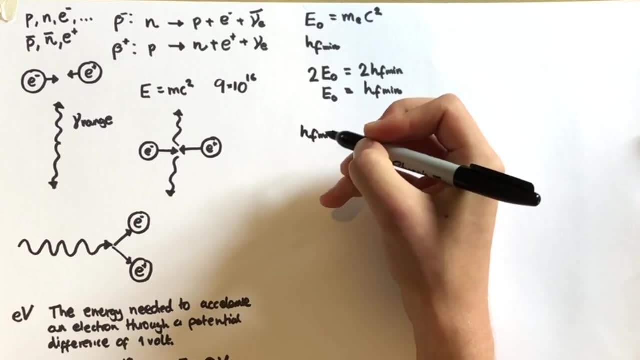 Now, with pair production, we have a photon which is travelling with an energy of h, f, min, But this becomes two particles which must each have rest energies- E naught. But since there are two, the photon actually has to have enough energy to produce two. 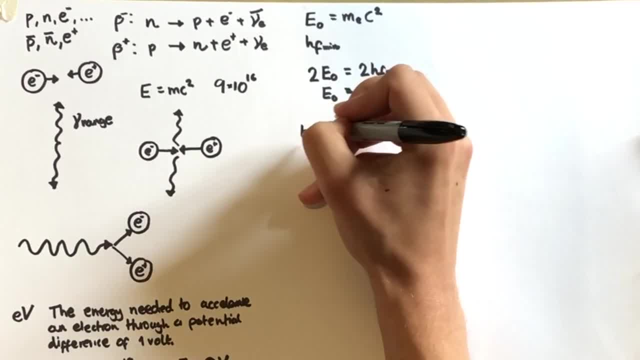 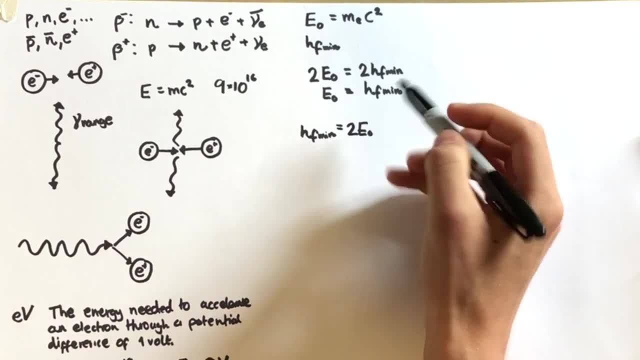 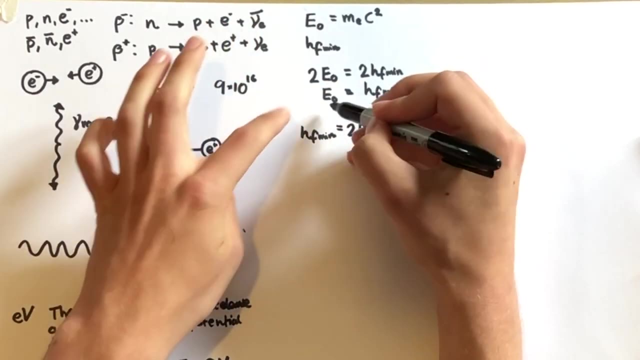 since you can't have a particle without an antiparticle. So therefore h f min in this case is equal to two E naught. So with annihilation the minimum frequency is just E naught divided by h. if we just divide both sides by h in this equation, Whereas with pair production 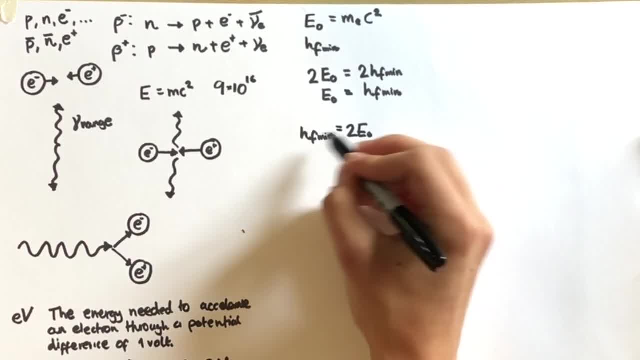 the minimum frequency is E. naught So with pair production, the minimum frequency is E. naught So with pair production, the minimum frequency is E. naught. So with pair production, the minimum frequency is two times E. naught over h. 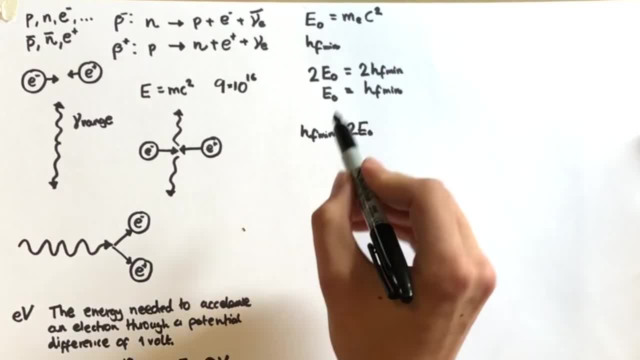 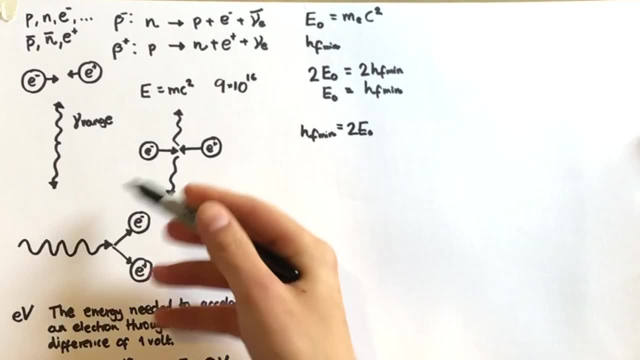 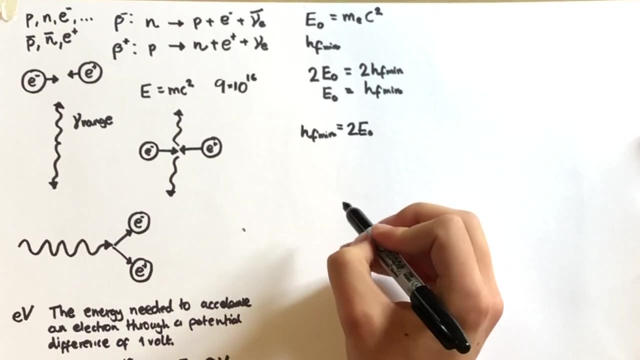 So you actually have to have a very, very a higher energy, a high frequency, moving gamma photon or gamma ray to produce particles. since you have to have the two, Any photon with less energy would not have the sufficient amount of energy to produce a new particle pair. 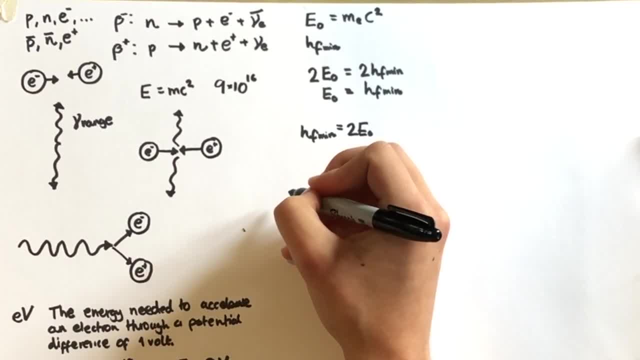 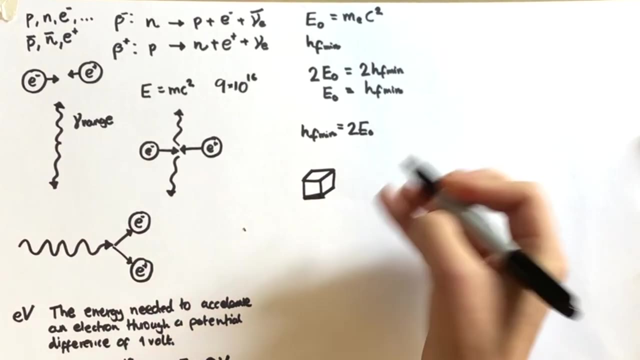 So now let's move on to particle interactions. So how do particles interact at this level? Now we know classically that an object, say we have a block here, this object experiences, experience many forces. you know it might have the force due to gravity. 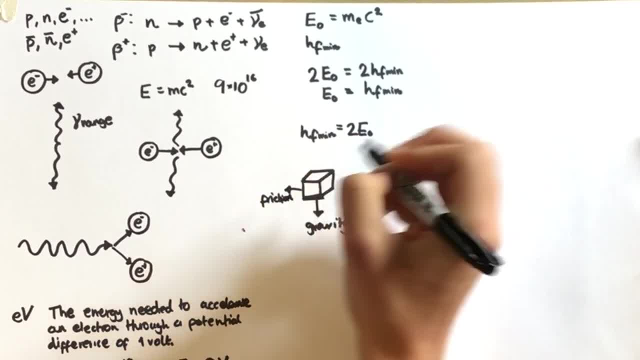 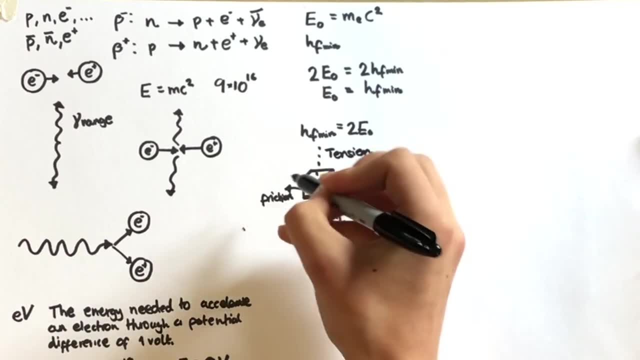 it might have some, might have some friction might be, I don't know. it might be hung from a ceiling, so there might be some tension in this, in this wire. We'll cover all of this in the section and you'll learn then. 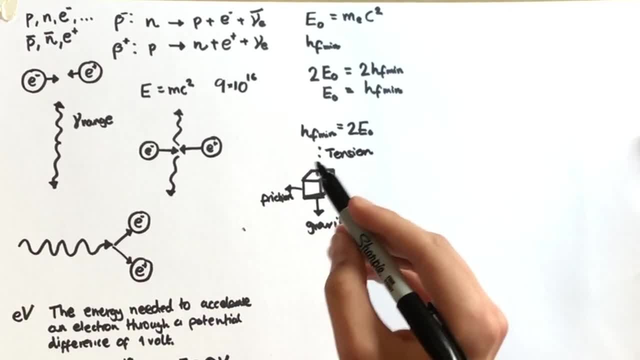 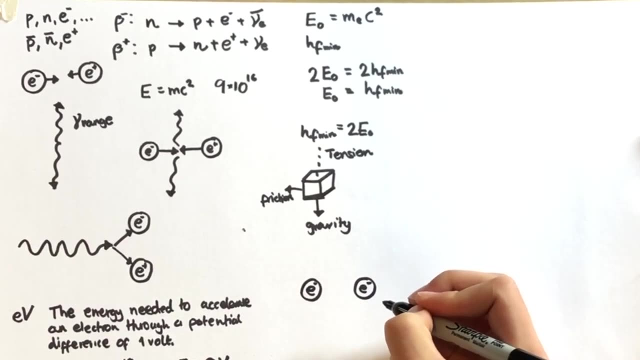 how to resolve forces. But this doesn't really apply at the quantum level. So how does it work? Well, let's say we have two electrons, So these are both electrons- E minus E minus. Now we know that electrons are negatively charged. 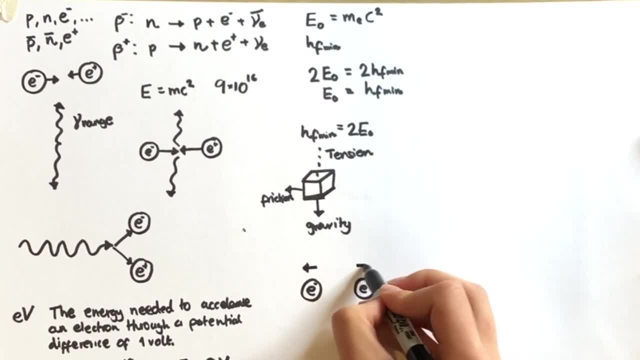 Therefore, there's going to be some kind of force that's going to repel these two electrons. Wijons, vayouts over why. And if we move from n to just x, if we're outside the quantum expression, there'll be functions. 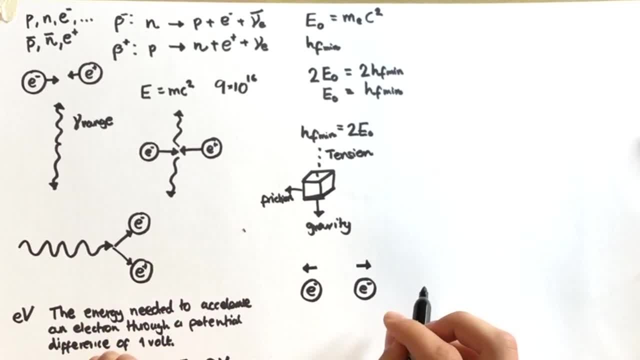 Oh wonderful, Let's just take on the dynamic Flip ready. Go on. So球 is an inflow. It displows it out from the center, from one another. But the question is, how do these electrons know that there's another one? 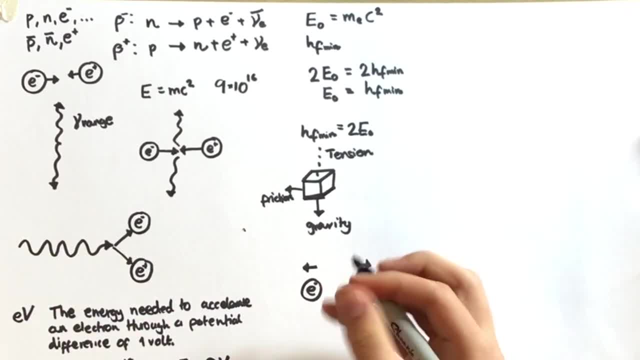 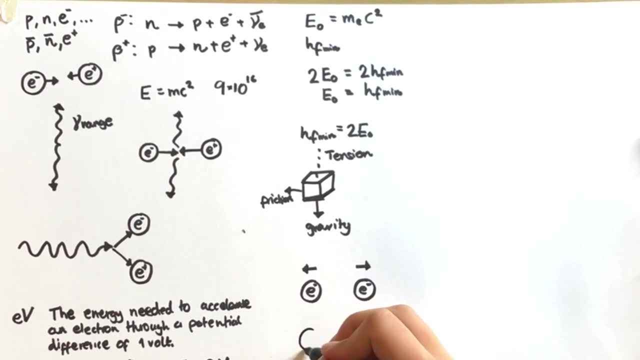 that's close by to cause them to repel. Well, it was the famous physicist Richard Feynman who worked out how this happens, and he said that between these two electrons- so these are the same two electrons- they actually exchange a photon between them and that photon lets the other electron know. 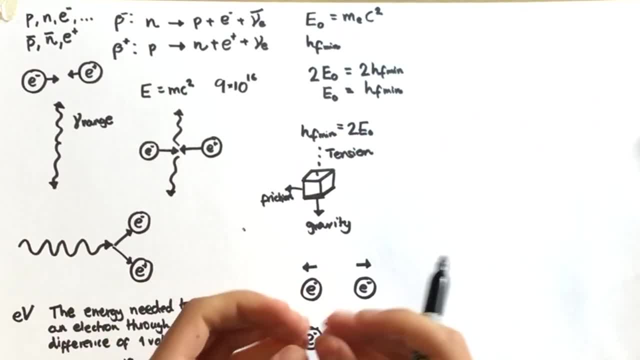 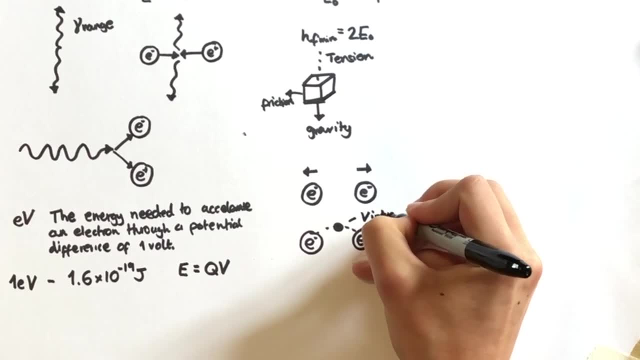 that it's there and therefore it knows to move away from the other. Now we describe this photon as being virtual, because we can't actually directly detect this photon. If we tried to, then we would actually prevent the force between the two electrons from actually 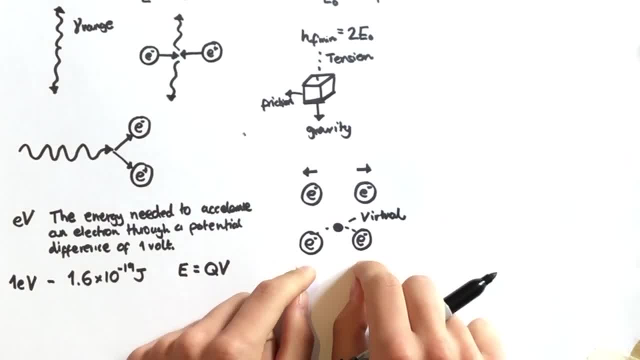 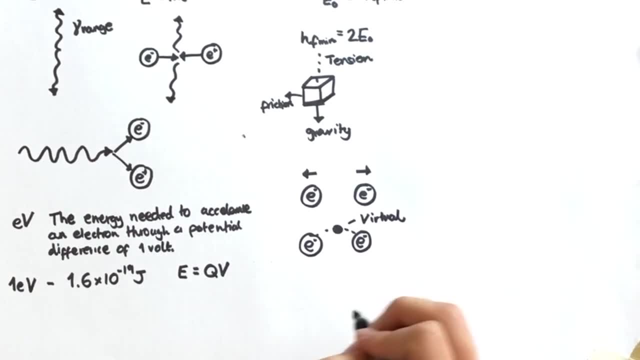 Now we can represent these interactions by what's known as a Feynman diagram, And you'll need to know how to draw Feynman diagrams in part as part of this course. So let's draw a Feynman diagram for two different electrons. 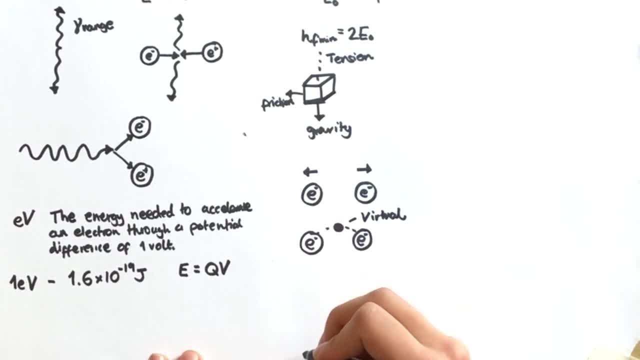 And as we do so, I'll talk you through the rules. So all incoming particles on a Feynman diagram all come in from the bottom. So in this case we have two electrons that are entering from the bottom. So we draw that. Now what's coming out of this interaction? 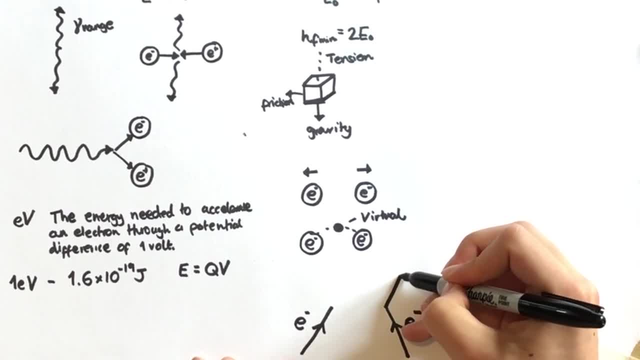 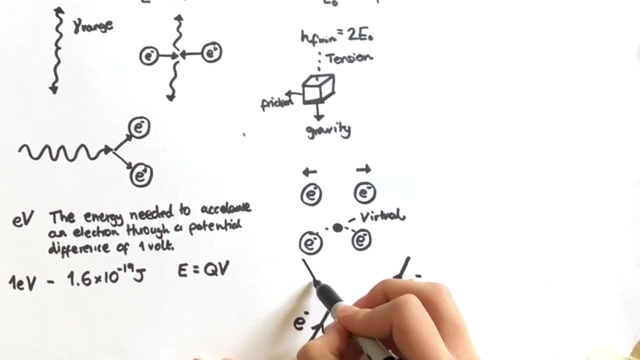 Well, just the same: two electrons. There aren't actually any changes in particles. In a second we'll draw What happens when there is a change in particles, But in this case we just get two electrons coming out. So two electrons coming in, two electrons going out. 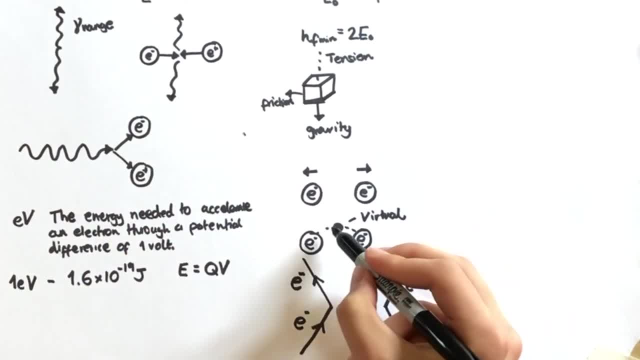 But of course we need to represent this photon right here, And this we represent by a wiggly line, just like this, And for the photon we normally use the symbol gamma, It's, it's just a convention. It's just a convention. 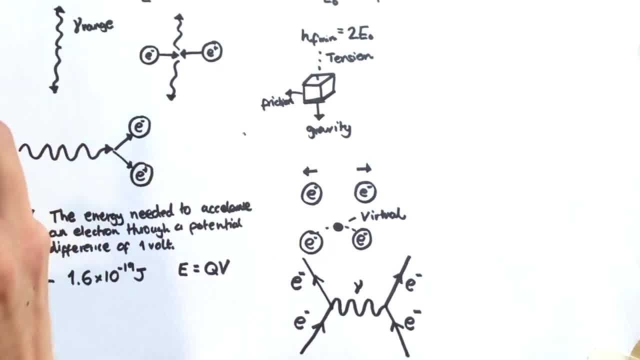 It's not necessarily this. It doesn't necessarily mean that it's part of the gamma, part of the spectrum, but we just normally use the symbol gamma to represent a photon. A little bit confusing, I know. So this is how, in principle, a Feynman diagram works. 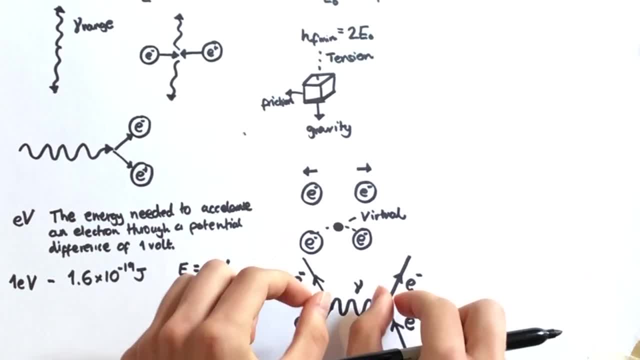 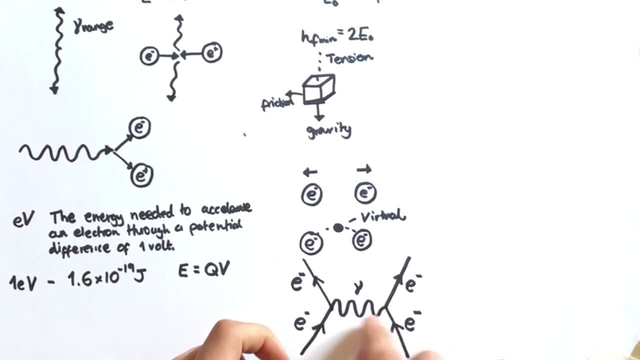 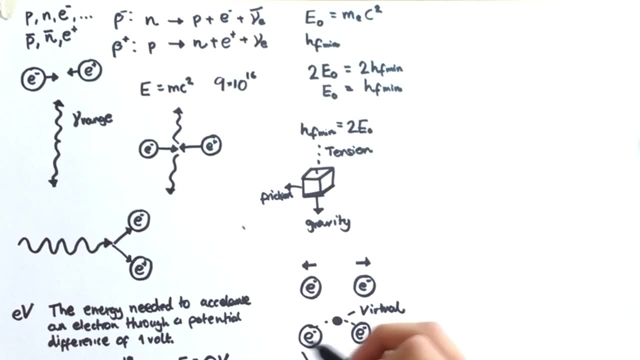 You've got the incoming particles coming in from the bottom, the outgoing particles coming out from the top, And you've got the interaction represented as a wavy line. Now this photon here represents the electromagnetic interaction between two electrons, But there is actually another force that's happening at this level. 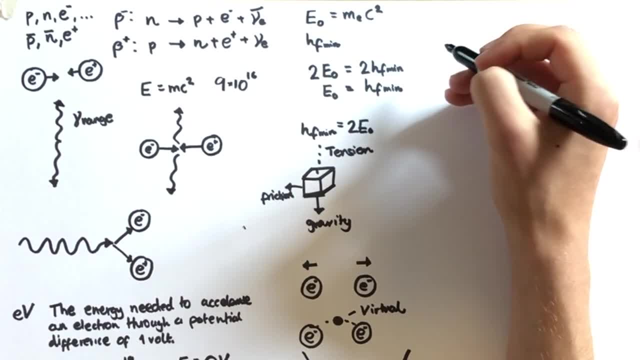 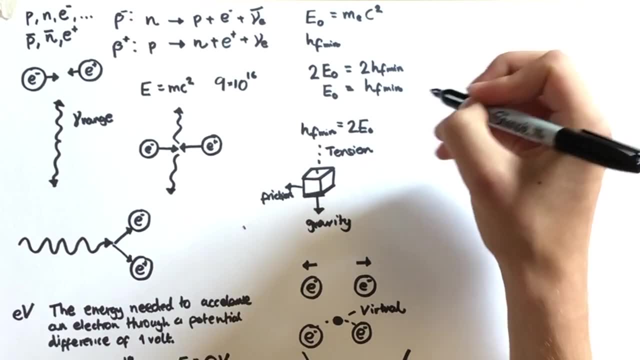 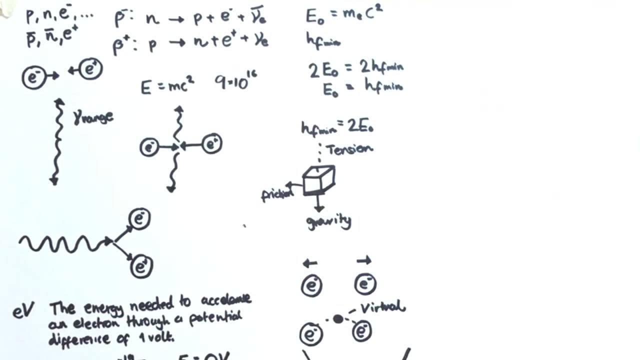 And we said before that there is the strong nuclear force that binds the nucleus of an atom together. But what actually causes, in beta minus decay, a neutron to transform into a proton? It can't be the magnet electromagnetic force, since the neutron is uncharged. 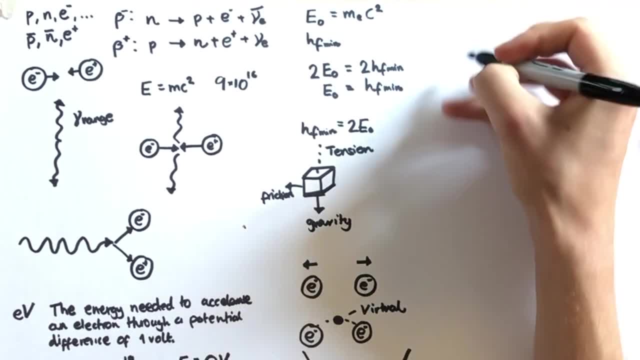 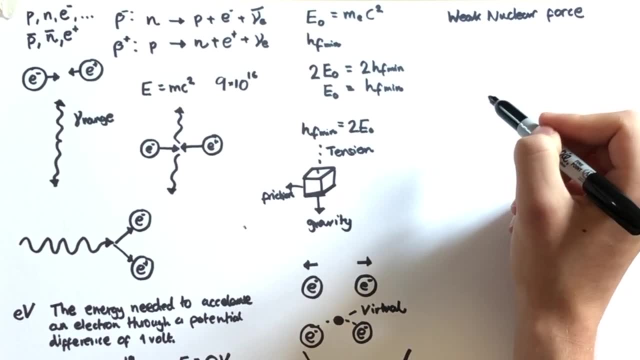 So there has to be another force at work. Now we call this force the weak nuclear force, And in beta minus decay and beta plus decay a new particle and a new antiparticle are created, But they're not a corresponding particle-antiparticle pair. 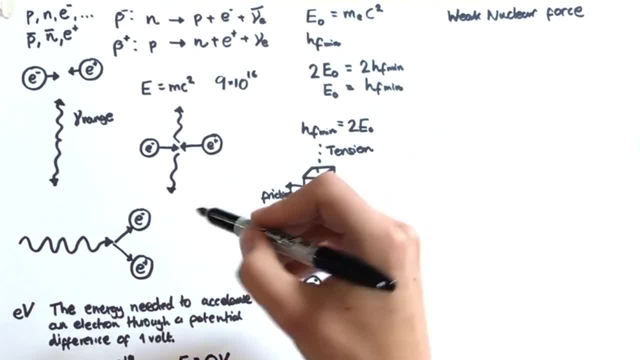 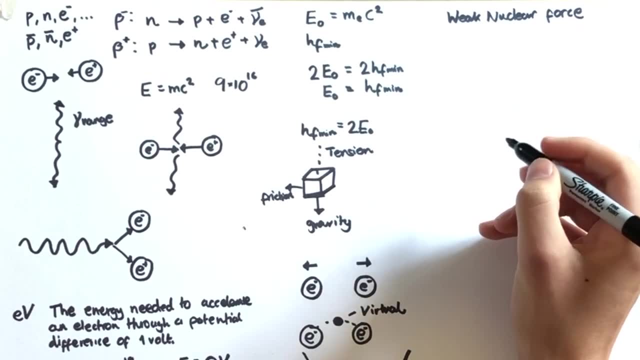 as one is an electron or a positron and the other is a neutrino or an antineutrino. Now, neutrinos hardly interact with other particles Since they have no charge, But you very occasionally get them to combine with protons and neutrons. 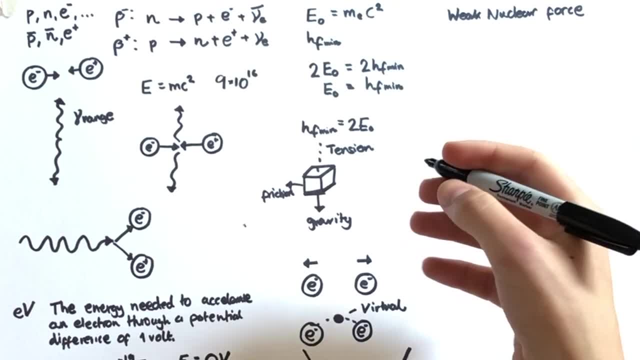 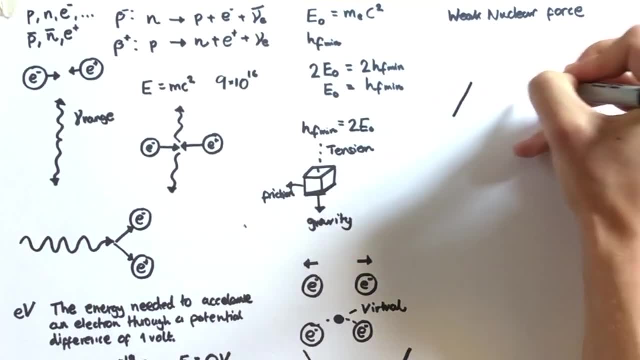 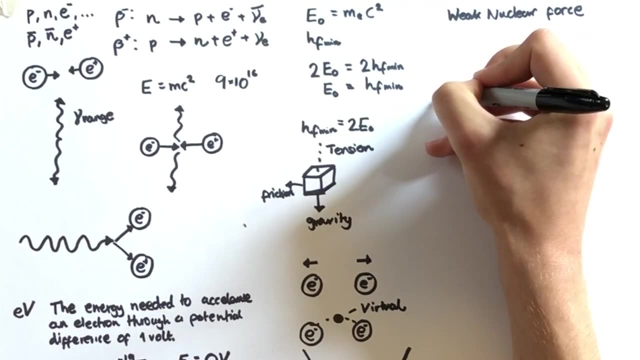 And we can draw this interaction between neutrinos and between protons and neutrons. So firstly, let's draw what happens when we have our two incoming particles. We've got a neutron coming in, We're going to do the neutron-neutrino reaction. 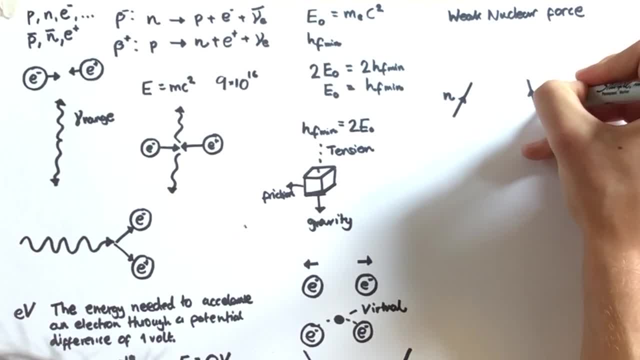 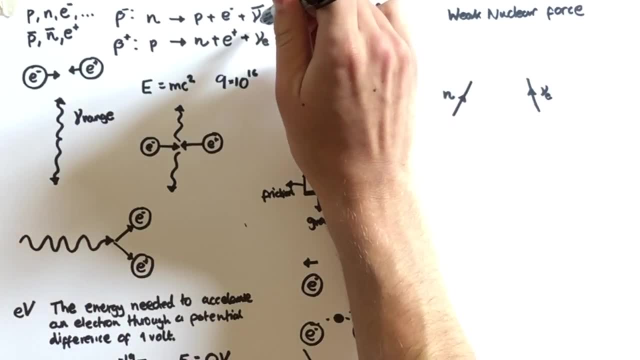 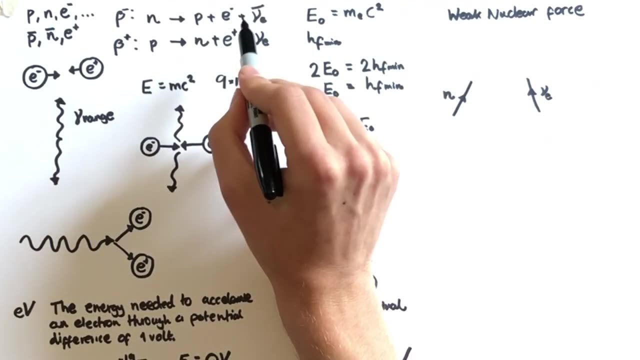 So we've got a neutron coming in, a neutrino coming in. This is an electron-neutrino. There's actually three different types of neutrino, which is why I've been using the subscript nu, sub e. This little Greek character here is known as nu. 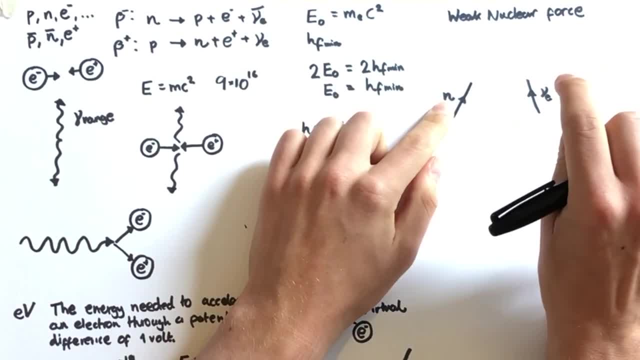 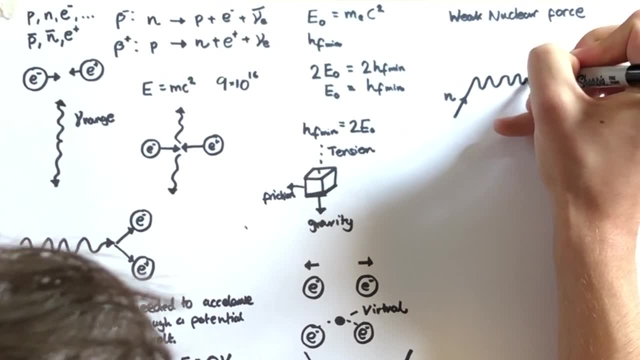 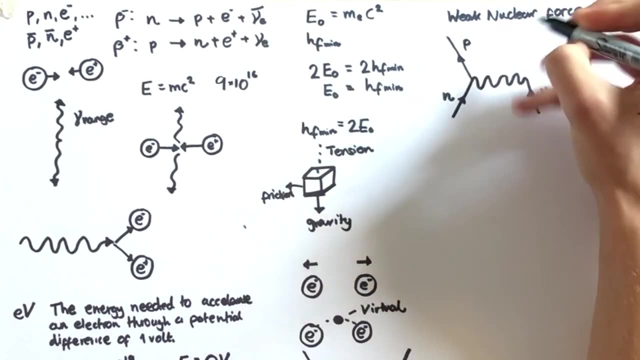 And so you've got the neutron coming in and the electron-neutrino coming in And they interact. And what do you get out of this reaction? Well, we get a proton coming out And we get an electron going out as well. 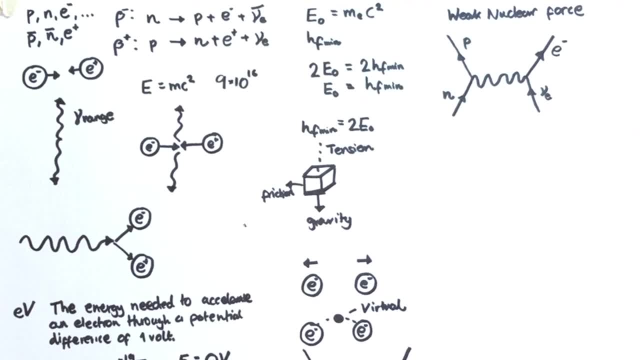 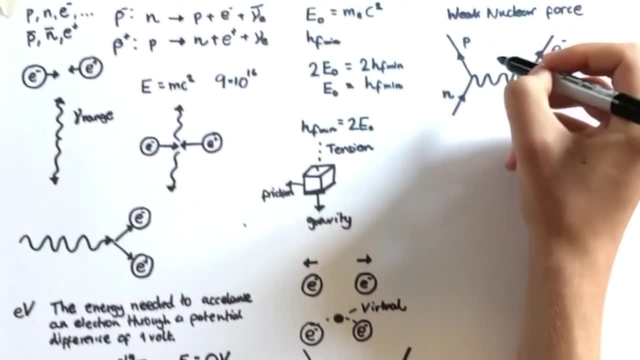 Now we said that in the electromagnetic interaction, the exchange particle, the virtual exchange particle, was the photon. But what is it, in the case of the weak nuclear force which is responsible for this interaction? Well, it's called the W. 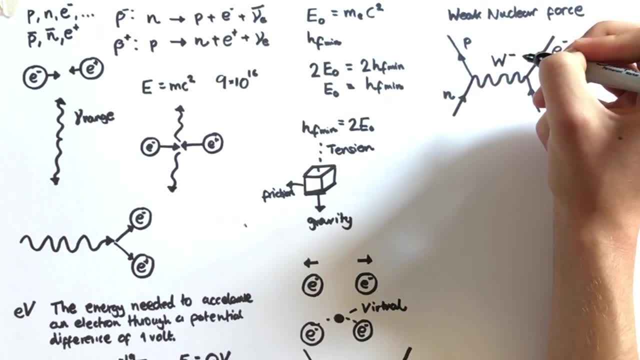 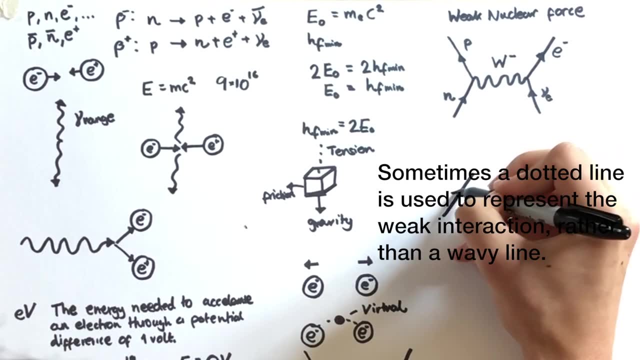 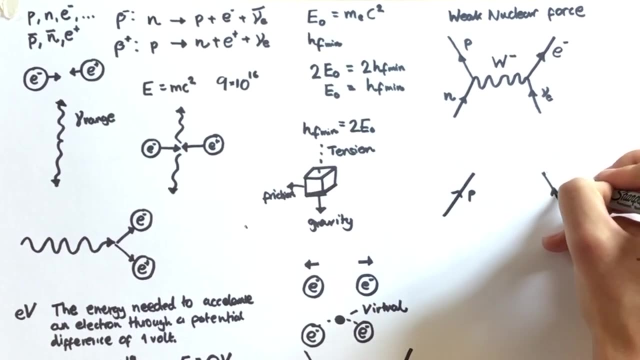 In this case it's the W minus boson. Now let's do the other, very similar interaction. This time we've got a proton going in And rather than a normal electron-neutrino we have an anti-electron-neutrino. 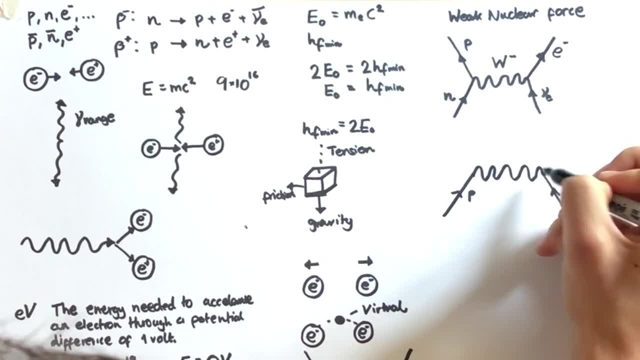 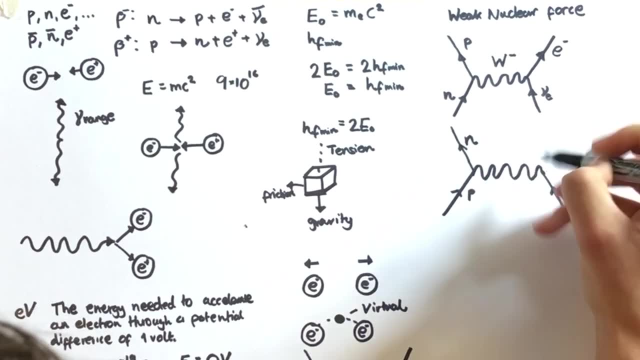 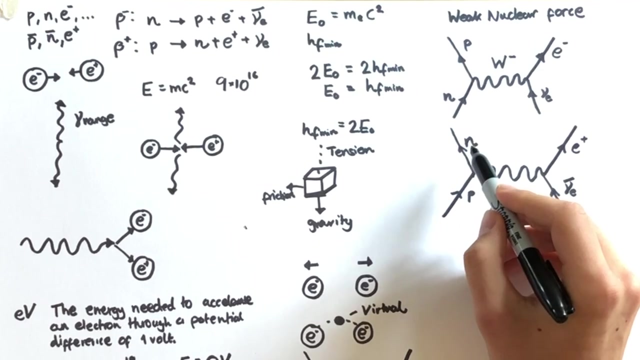 And they interact a bit like this: And you have a neutron Coming out And on this side you have a positron coming out. Now notice that all protons and neutrons, which are actually collectively referred to as baryons, 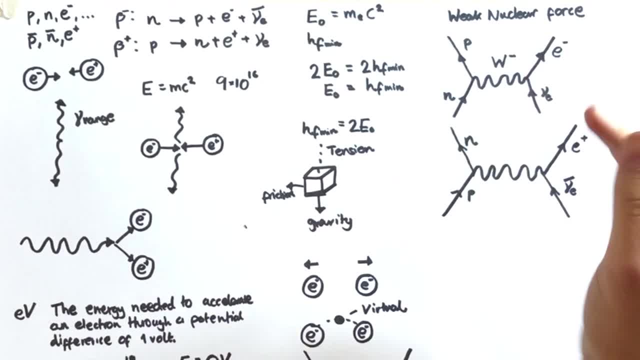 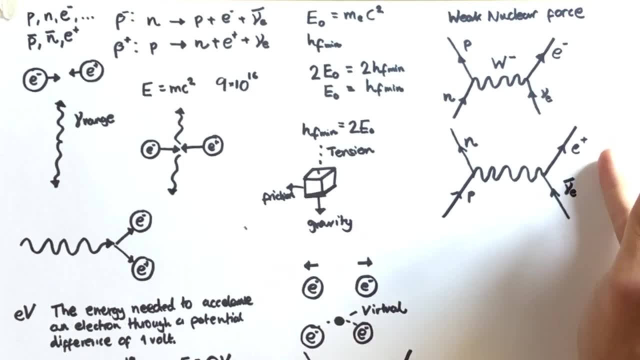 we'll come onto this a little bit more later- are all on the left-hand side, And all of these guys right here are leptons, And they're all on the right-hand side, And this is a convention used with the Feynman diagram. 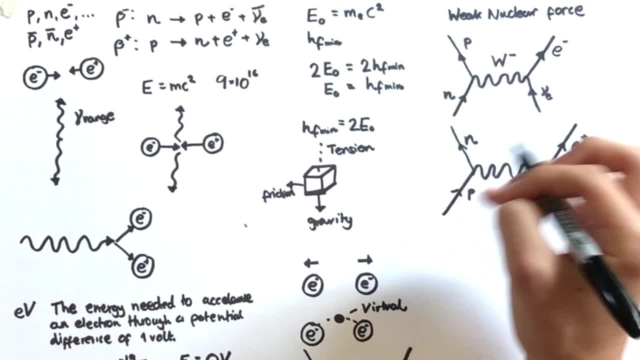 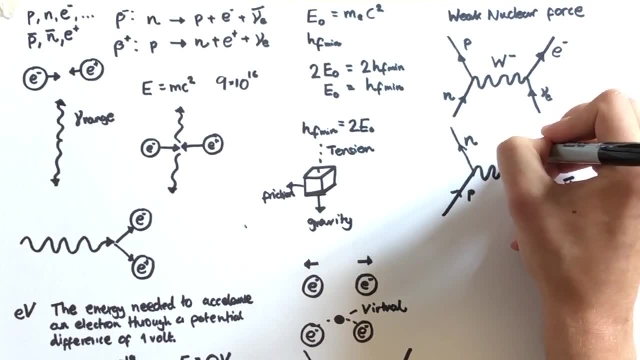 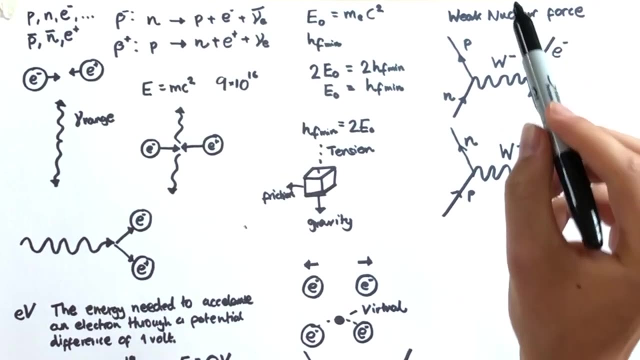 But we'll go over all those definitions in a lot more detail when we cover that, And instead of the W minus boson causing this reaction, we have the W plus boson. So what are these W minus plus bosons? They're the exchange particles responsible for the weak interaction. 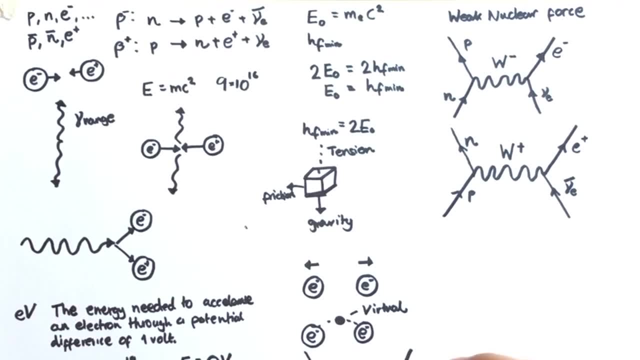 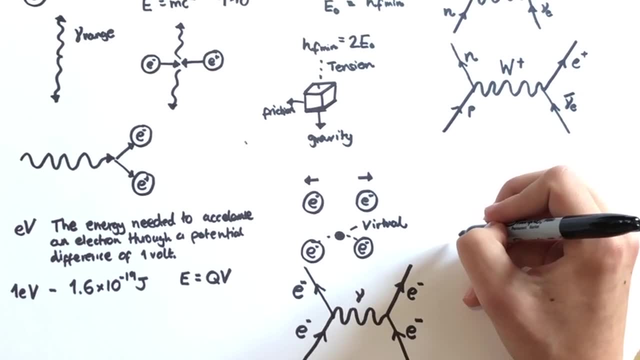 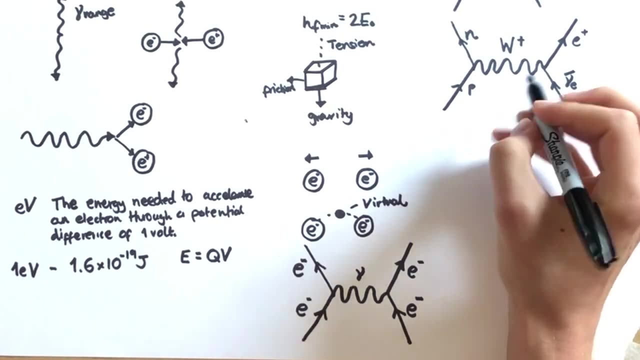 Now, unlike photons, which have no mass, these particles are very heavy, And so they have a much, much shorter range. So I'm now going to draw out two more interactions, And this time I'm going to draw out the beta minus and the beta plus reactions, using this. 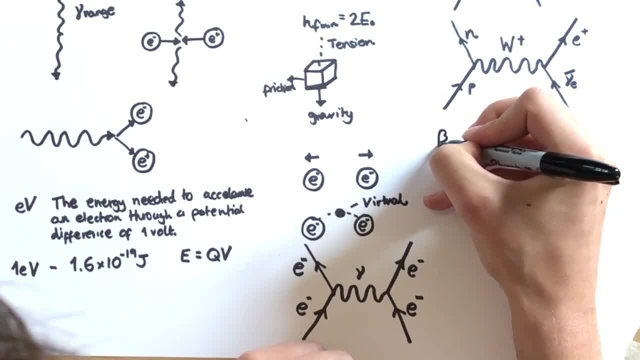 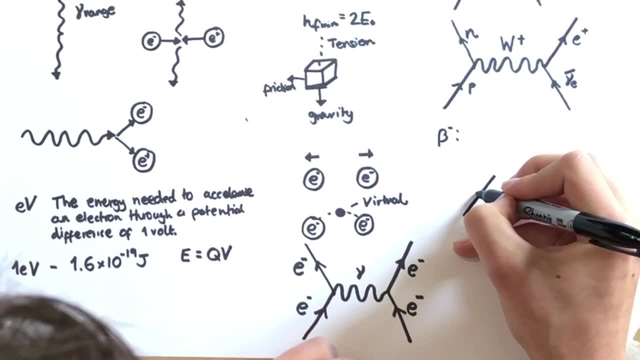 Now that we know the force responsible, we can draw out the beta minus and the beta plus. So let's start with the beta minus interaction. This is probably one you'll have to know. So we have the beta minus, We have a neutron. 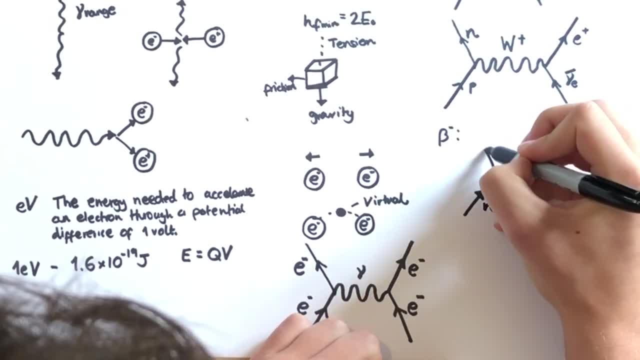 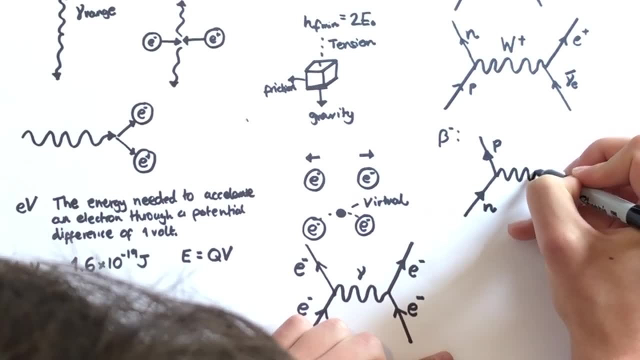 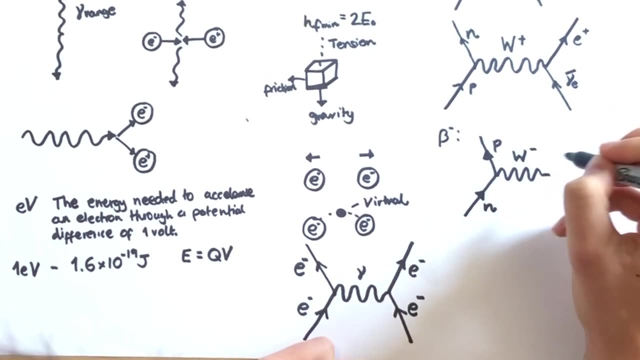 We have a neutron going in And what's going out? We have a proton that's going out And they interact via the W minus boson. in this case, The easy way to remember it is: a W minus boson corresponds to an electron going out. 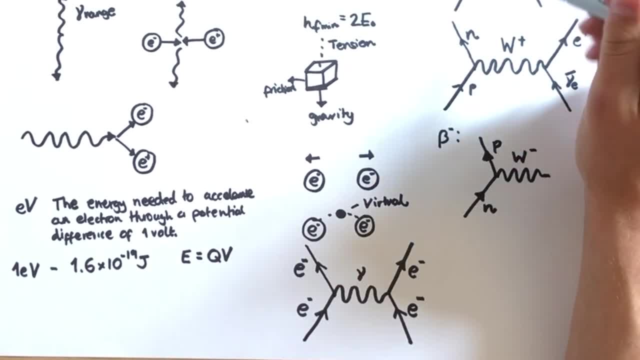 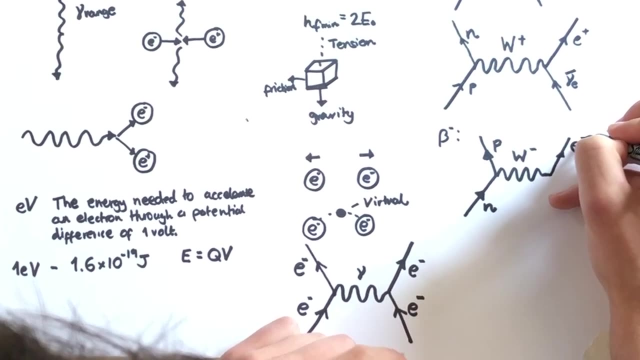 And if you have a W plus boson, you have a positron going out. The sign of the W boson is the same as the sign of the electron that's leaving, So that's an easy way to remember it. So you have the electron going out like this: 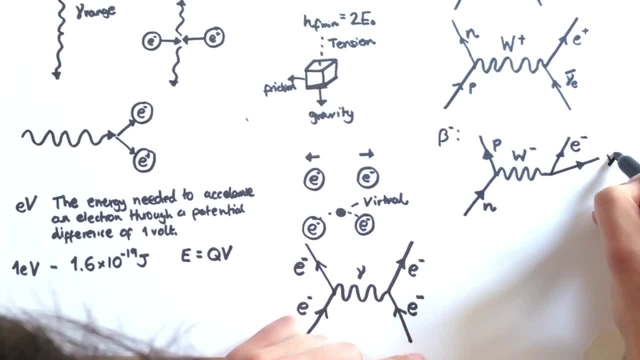 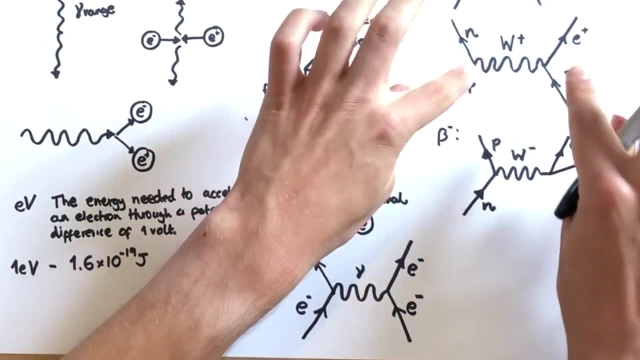 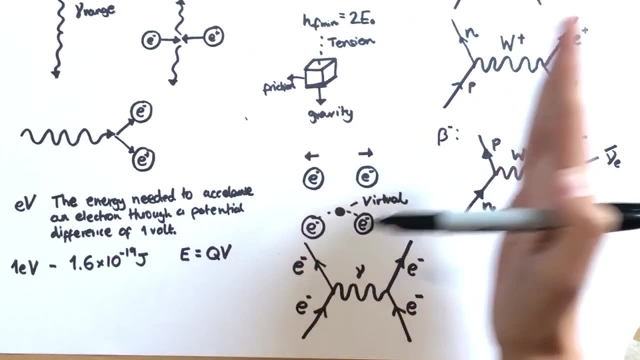 But of course we also have the anti-electron neutrino. that's also going out. So you see, all of these particles are going out. So, rather than having two in and two out, you have one in and three out, But because of course you have baryons on the left and leptons on the right. 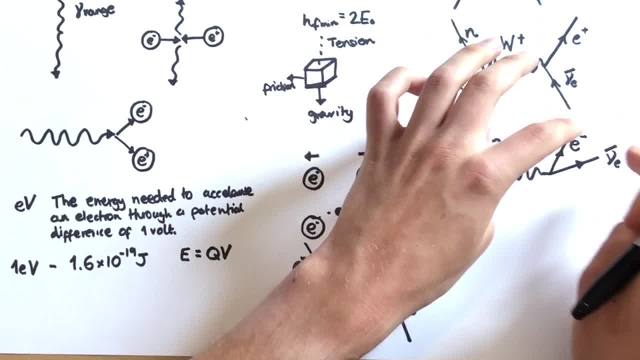 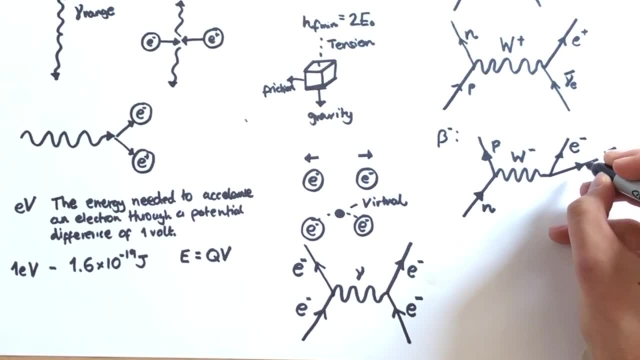 then protons on this side and the electron and the anti-electron neutrino are on this side. Now, technically I'm not sure whether they're that fussed about it, But because this is an antiparticle, there is a convention that you should technically draw the arrow going that way rather than that way. 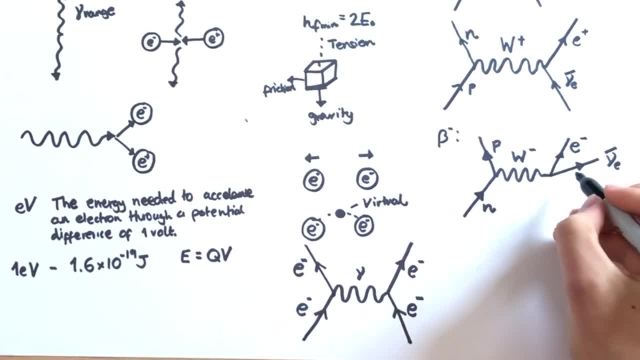 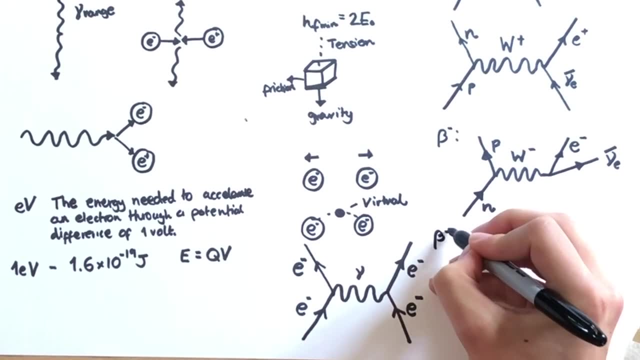 Now this is something I don't know if they're too fussed about, But technically that would be the right thing to do. So let's just finish this off. Let's do our Feynman diagram for the beta plus decay. 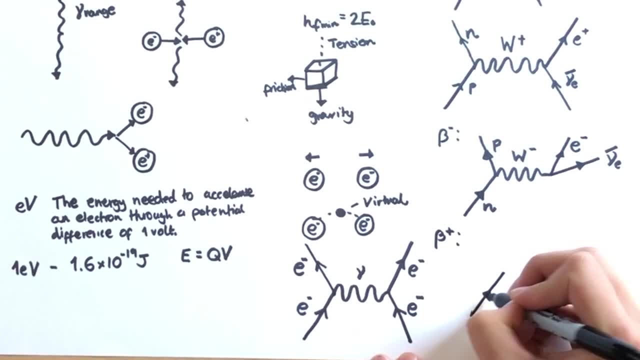 So, rather than a neutron turning into a proton, we have a proton turning into a neutron. So there's all our baryons on the left, Here's our little wiggly line, And we have W plus boson, Which is the exchange particle responsible for this reaction. 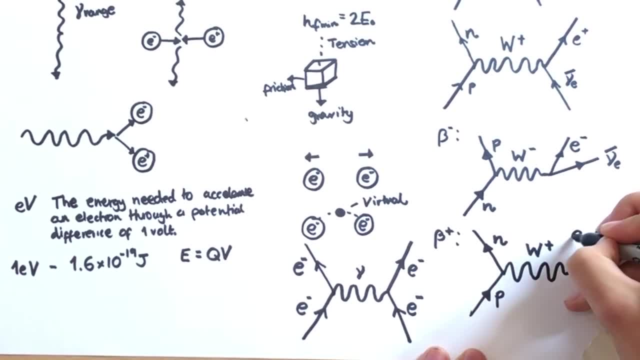 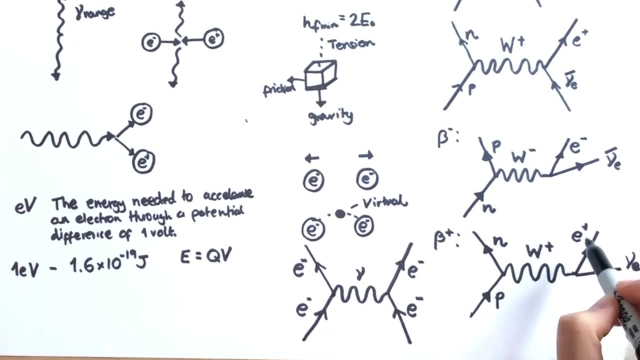 And we have our positron leaving, As well as our normal electron neutrino And again, technically, this arrow, because it's an antimatter particle, the positron. it should be technically going in, But again, I don't think they're too fussed about that at A-level. 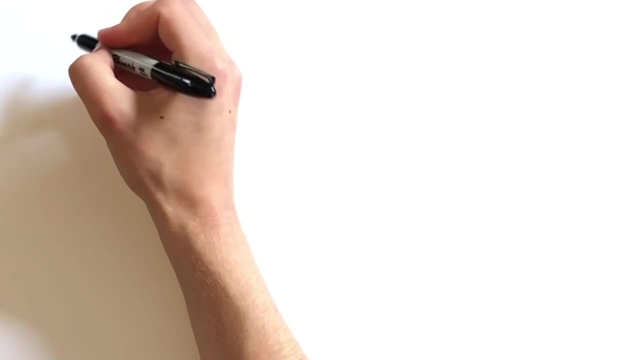 Now there is also a final type of interaction involving the weak interaction, And this is known as electron capture. So before I do the Feynman diagram for it, I'll just do a brief schematic of what it actually is. So say, you have a nucleus right here. And this nucleus is normally proton rich, So it doesn't have enough neutrons, but it has a lot of protons for the given number of neutrons. Now what it's going to do is it wants to convert all these excess protons into neutrons. 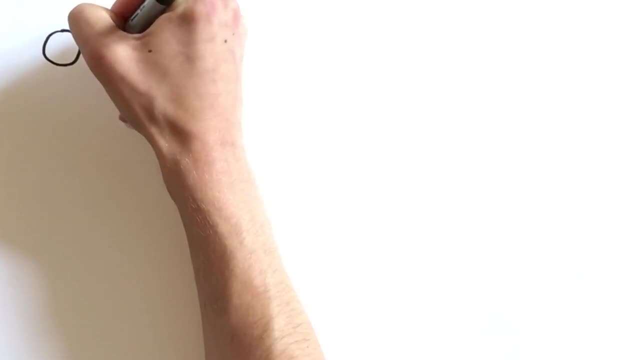 So how's it going to do that? Well, thankfully there are lots of orbiting electrons And we know that when we combine protons and electrons we get neutrons. So here's a proton in the nucleus And here's the electron. 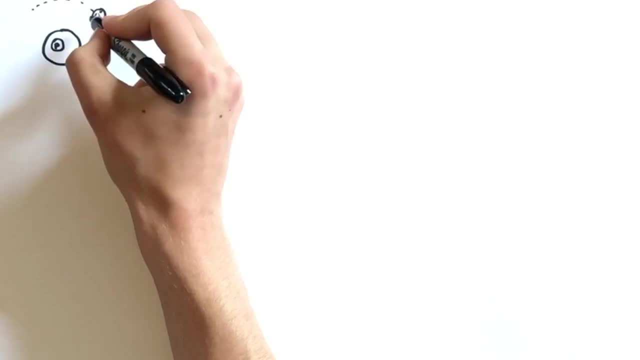 This nucleus will literally capture the electron from the nucleus, From the shell that it's orbiting in, and create a neutron And this will normally spit out an electron neutrino. So let's draw a little diagram. So in the bottom we have our proton that's going in. 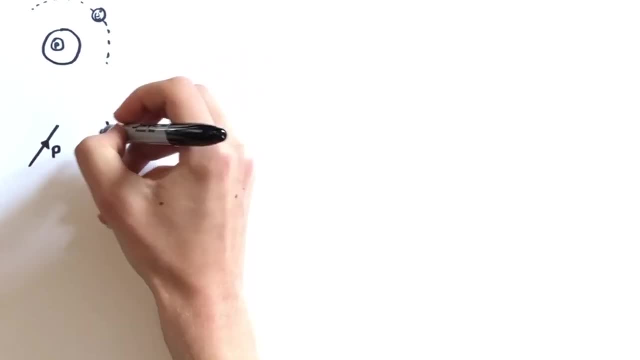 Protons are the reactants in this case, And you have the electron that's orbiting. So remember, leptons are always on the left Now, because the electron is actually incoming rather than going out. it's the W plus boson.